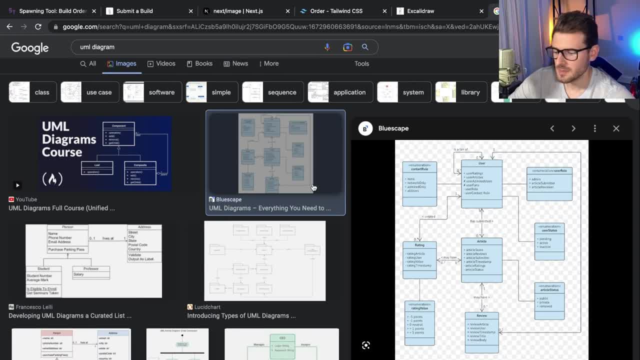 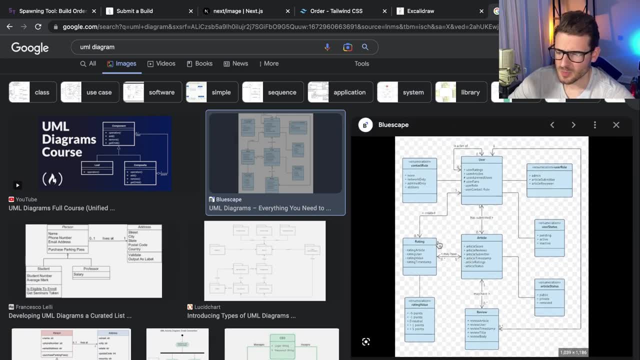 database and you want to set up some entities and some schemas. Some people sit down and they'll draw out this huge diagram of all these entities, how they interconnect, which is cool. but it's a very waterfall type of approach to software engineering And, from what I've learned, or where 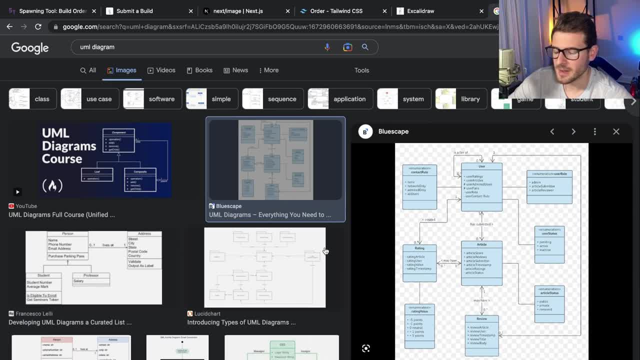 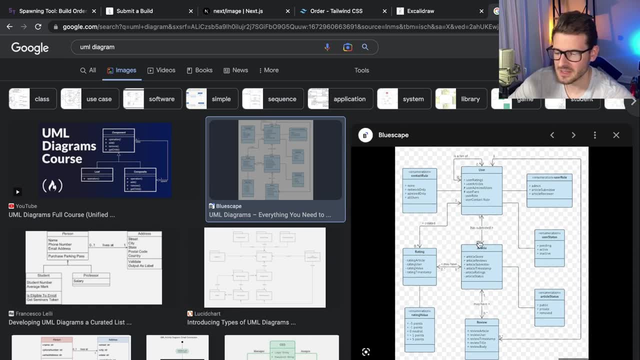 I work and, like the mindset that I have is I like to try to work in an agile mindset. So basically, instead of sitting down and trying to design out the diagram of what every single entity might look like, for example, in this application I'm building for a 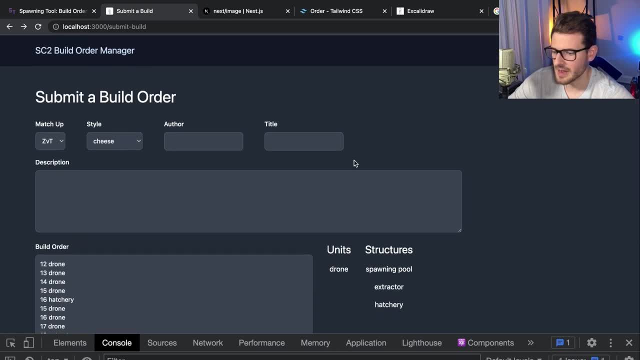 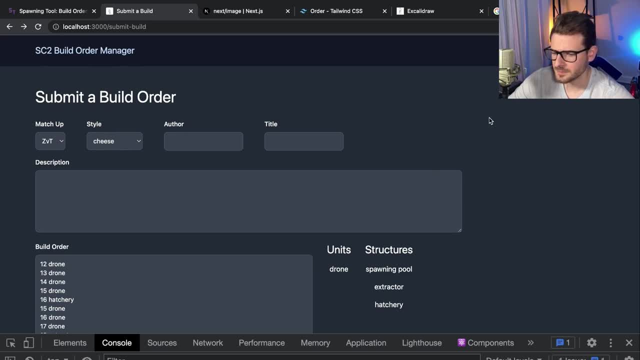 interconnect and how they do this and that and the other, But what I found to be most beneficial to me is that start on one single thing that helps you implement the feature that you need right. That's like the agile mindset of do the bare minimum that you need to do to actually create. 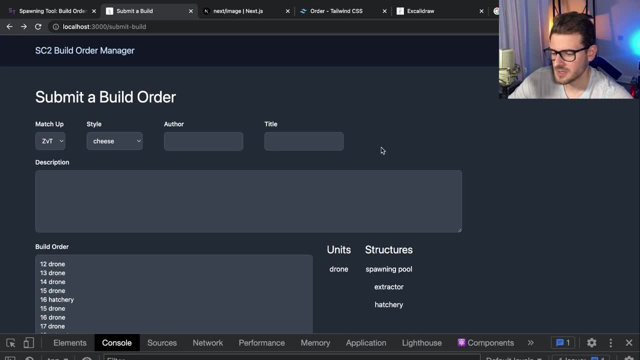 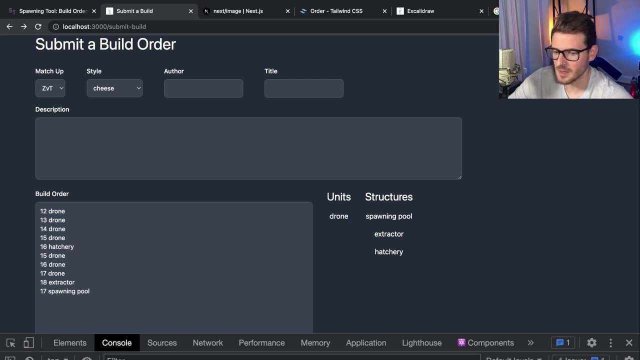 a feature for your users. Now, the reason that I like to do that is because most of the time, you don't know if what you're building is actually going to be useful for the users that you're building it for. you may spend weeks or months designing this giant system. you have all these. 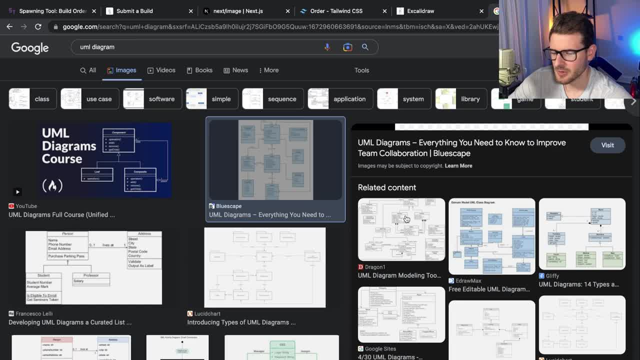 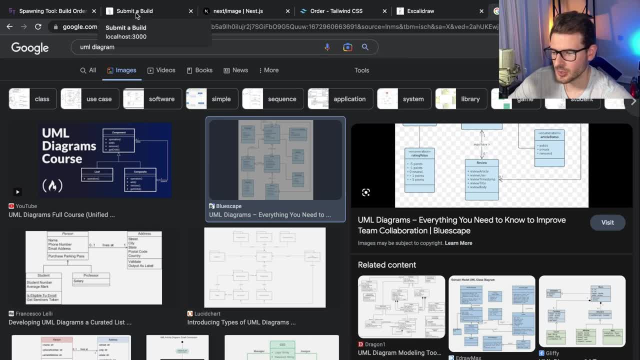 nice diagrams with arrows and stuff, and then you start coding it up and you realize that everything you designed is completely wrong, or it's not going to work, or it's just not fun to use or it's not good to like be maintainable in terms of the long scale projection of your system. so i try to avoid. 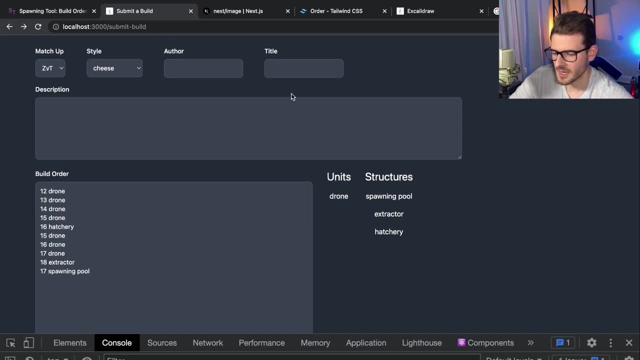 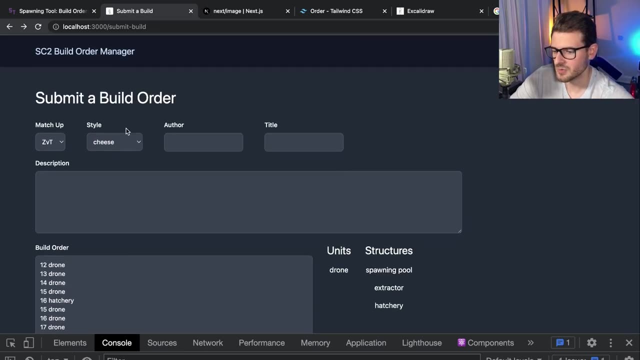 diagramming. now, if you get a feature where you need to like do something, where like, for example, let's say, they create this build and you need to have that, send out an email and also send out notifications to people who might be subscribing to you as a user, then, yeah, i might sit down with. 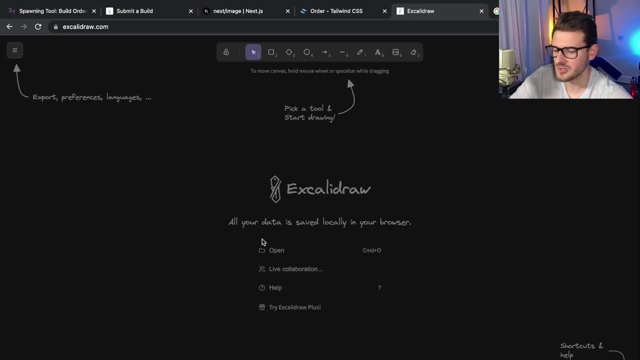 excella draw and i might start diet like diagramming out like what happens, how does the flow of code happen for this particular feature? but i'm just focusing on that one feature i'm trying to add. i'm not going to go off and start like adding all these different pieces to the puzzle, especially. 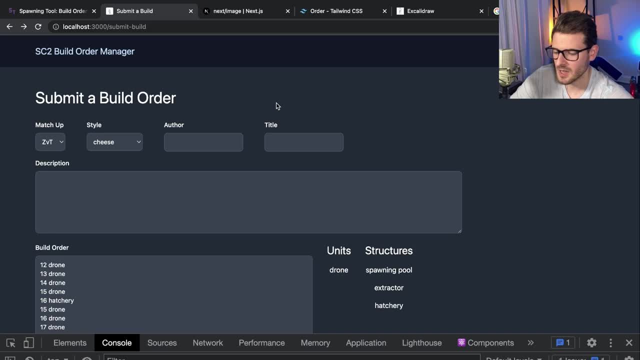 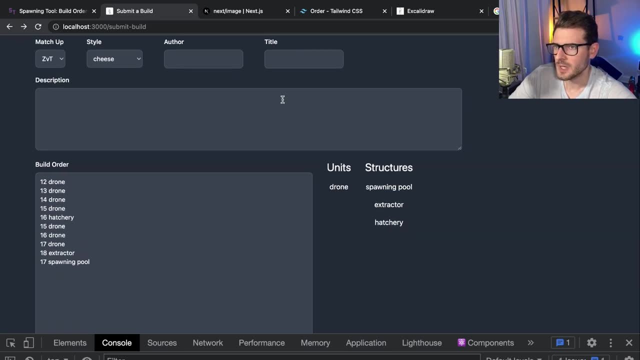 since if we're not focused on building that feature yet, then i would not waste time thinking about that feature. and this does have some drawbacks, because sometimes you you need to stick a step back and think about the bigger, the bigger pieces, like you need to holistically look at what you're building. 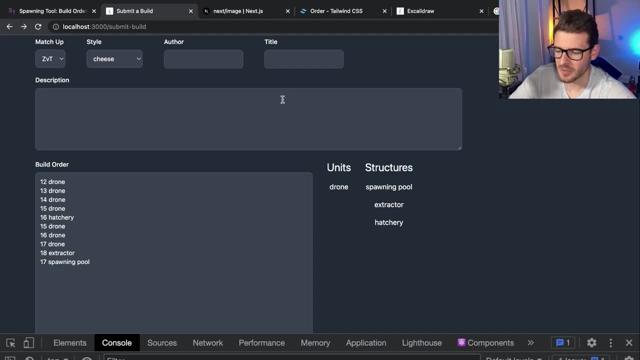 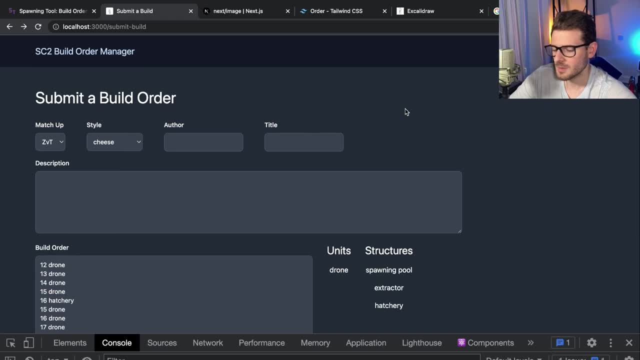 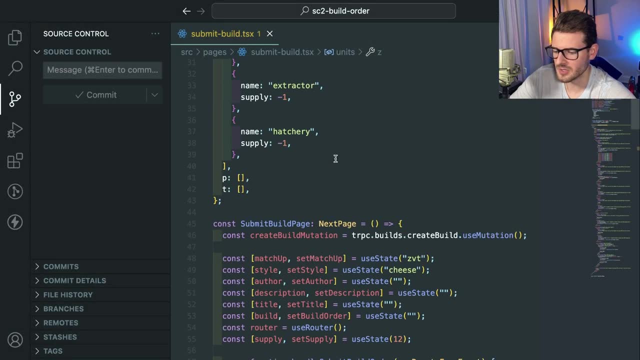 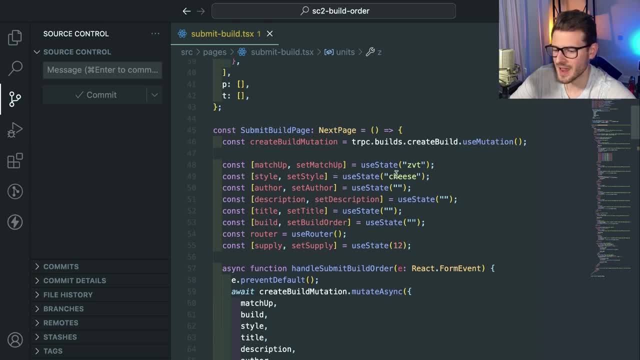 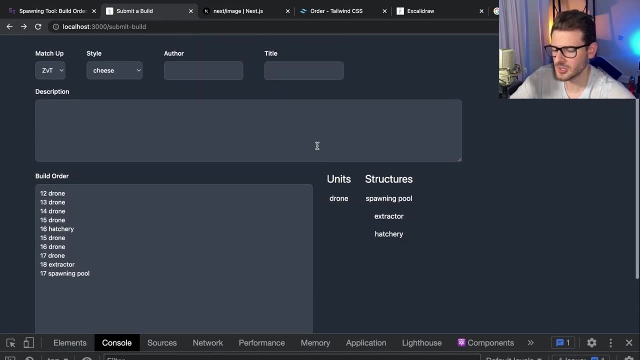 your code base that you may or may not even need, right. so don't add things to your code unless you know it's going to achieve the feature that you're trying to build out for the user, and i like to do this step by step, so every feature along the way you continuously iterate, build upon the feature. 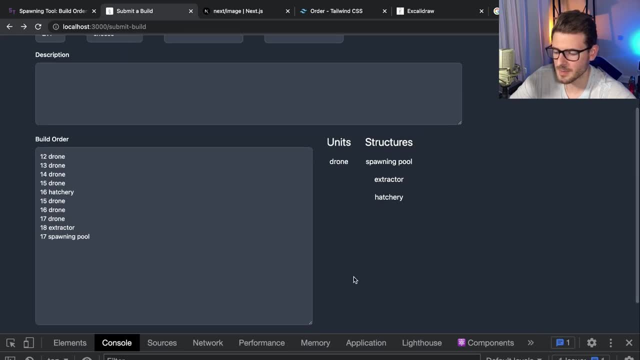 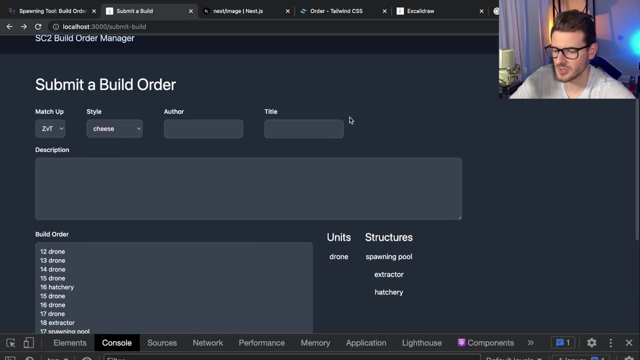 and i'm not saying that the code you write has to be sloppy- like you should be shipping quality code. you should have tests that cover everything you write. you have integration tests, unit tests, end-to-end tests. you should make sure your code, you know, follows proper coding standards. like you. 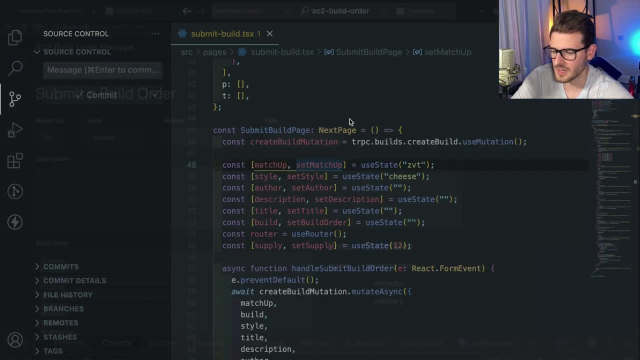 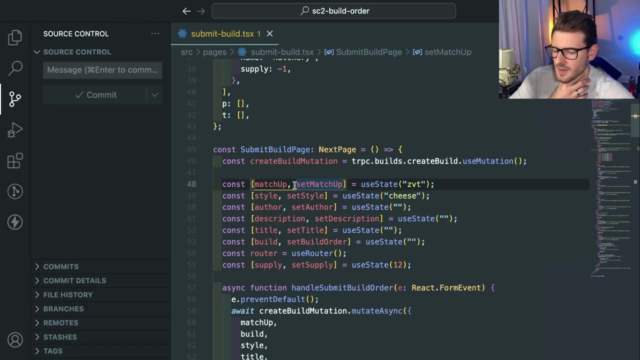 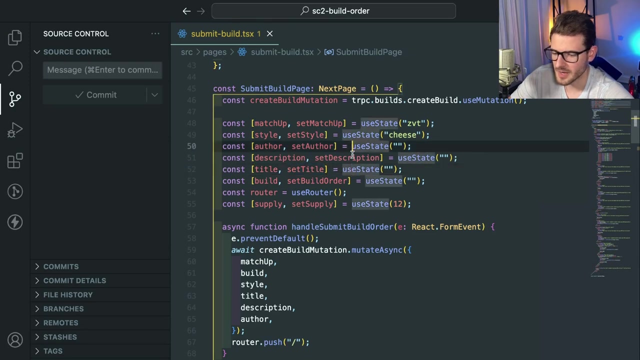 know clean code. you have your magic numbers removed, you have any constants pulled out to a shared location. um, you know, stuff is documented, stuff is commented, but i'm not. but what i am saying is like, don't try to add in a bunch of additional things into your code for the what ifs right, you don't know what the user. 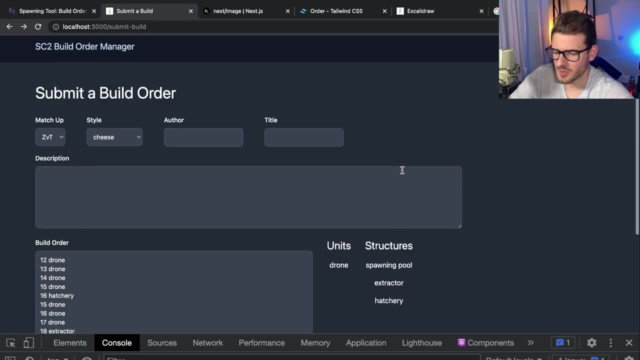 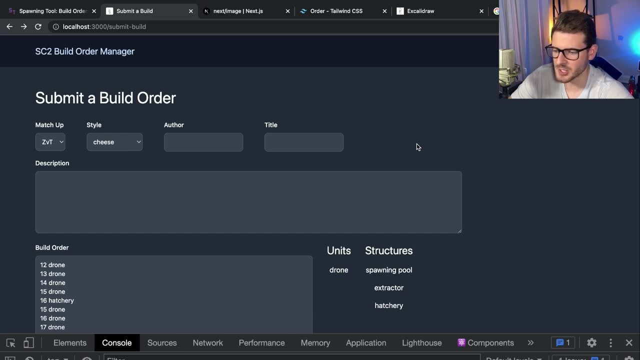 needs in the future, so don't try to code for that. so that's kind of the approach i like to take in the way that i've been kind of taught um with where i work and like, since i started in the industry, to have an agile mindset of just build one feature and then ship it, get it out there in. 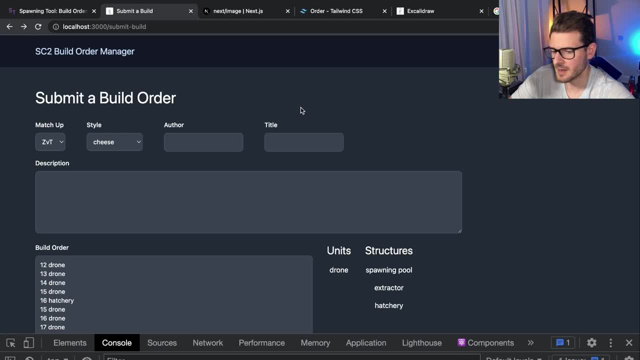 front of users so that they can play around with it and they can give you some feedback. even if you have, like, a feature flag that basically only lets certain subset of users to use this new feature, it's more important to have a certain subset of users to use this new feature and 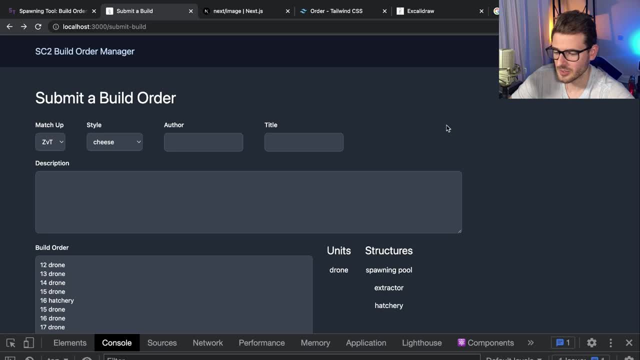 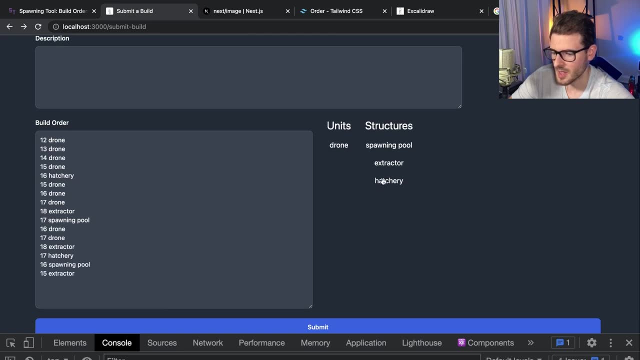 it's more important to get this in front of like a test group of people so they can say, hey, you're wasting your time. building this like this is not what we want. we do not want this ability to basically create a build order for starcraft 2 by clicking on buttons. i'd rather just go in and 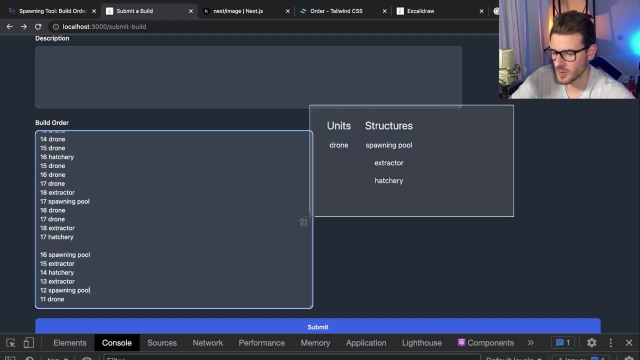 manually type stuff if that's what your users want, then you don't have to spend weeks building out this feature that no one would ever want to use and then also polluting your code base with a bunch of stuff that you're just going to end up deleting or just let sit around and rot that you. 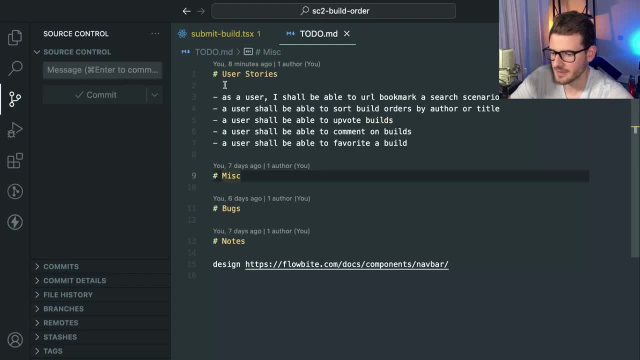 don't want, and so that's kind of like the way i do things and i'm going to show you how to do that. like i kind of start with a single user story, like, for example, in this build order project i'm building that's, that's using the t3 stack with like prisma and next and stuff. i basically just 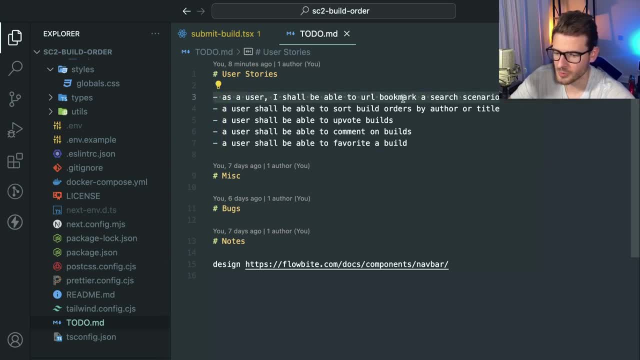 write down a single sentence like: as a user, i should be able to url bookmark a search scenario and all the stuff that comes after. that is all like implementation detail. that's not really important and i just work towards implementing whatever that feature is and then, once i'm done, 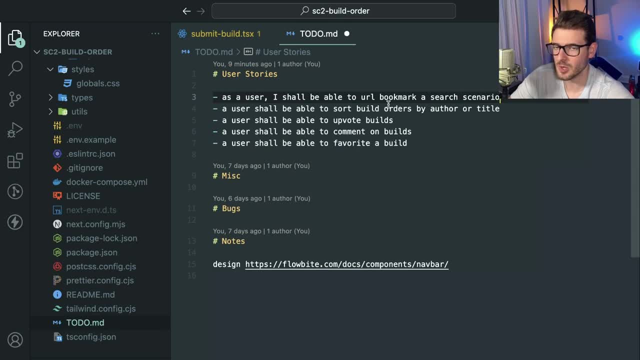 i will just commit that and then hopefully your cicd pipeline will automatically deploy that to your users. they can start using it and they can give you feedback and then you move on to the next user story. so that's kind of like the agile mindset i'm obviously i'm kind of boiling. 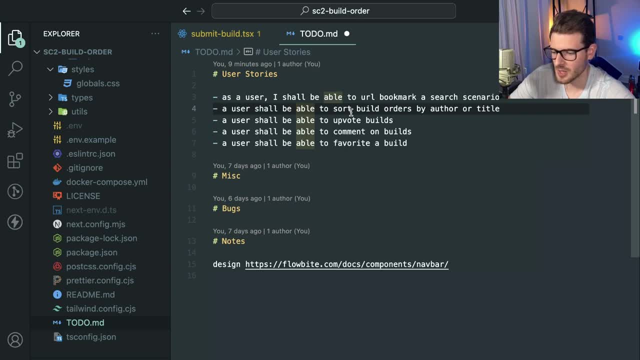 this down to the most basic um explanation. there's a lot more that goes into it with, like, the planning and the orchestration of your stories and actually deploying these things and testing them. but overall, if you're working on like a side project, i like to just do this, just write out. 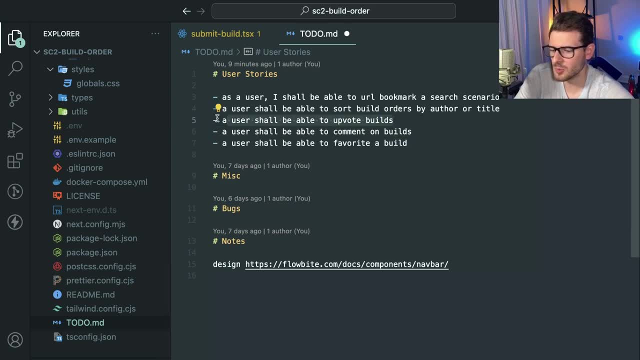 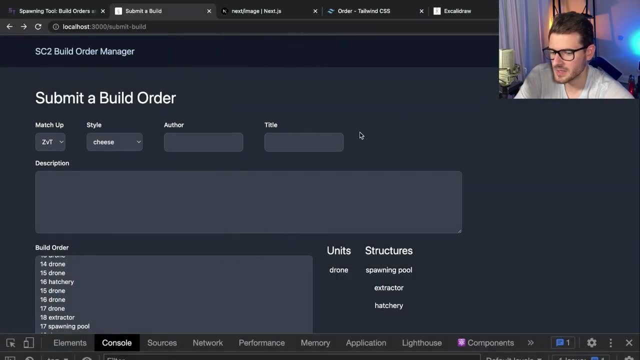 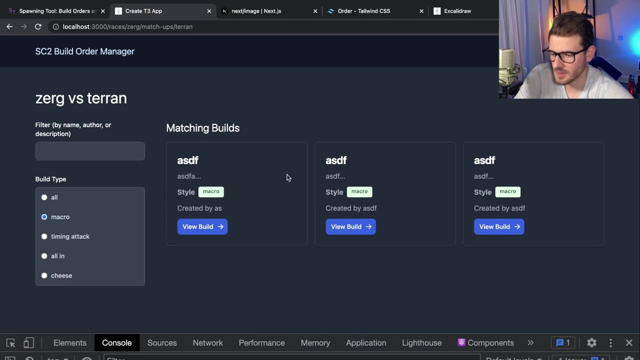 a simple feature and add the most minimal amount of code that you can to make this feature work. like, for example, a user shall be able to upvote builds. well, if i wanted to add that basically, i would just go and find a single area like: maybe it's here, maybe you want to be able to upload. 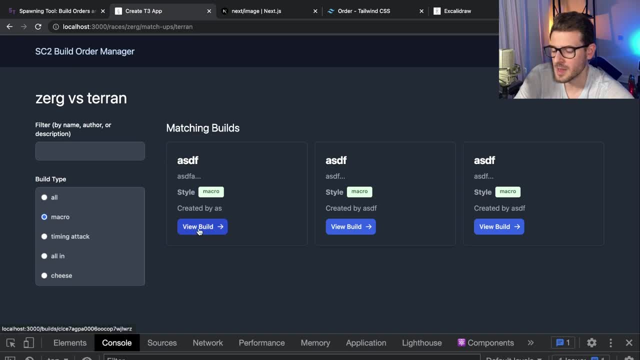 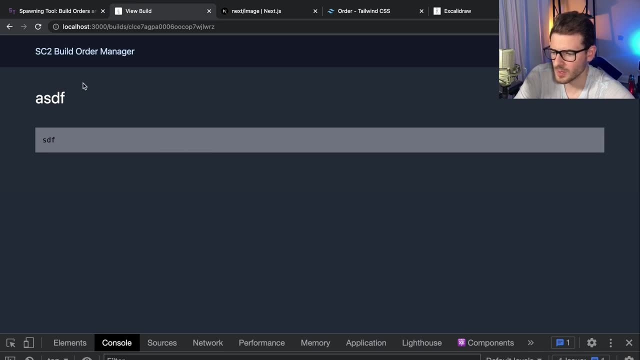 upvote builds from this little card component, or maybe you have to go into the build itself to upvote and you don't know. like the good design, you won't know if it works, if it works better here, works better here, or works better on both pages, until you actually get into the 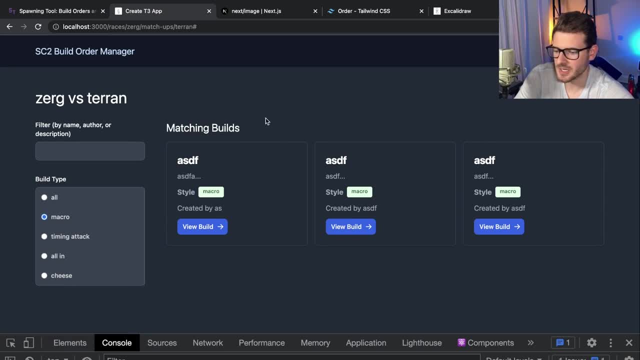 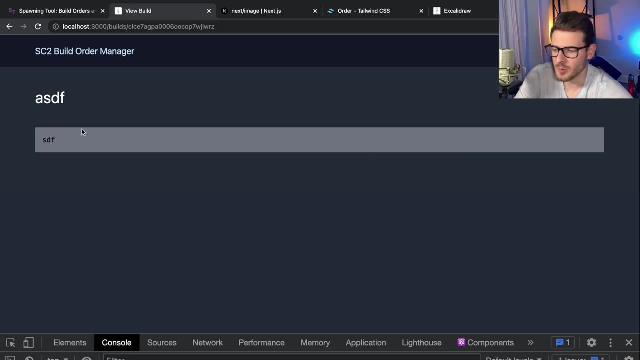 weeds of the implementation and start adding it in and start using it and you realize, okay with with like analytics and tracking on your app, you notice that only five percent of users are actually up voting builds on this page. so if you have it here and you have it here, you're kind of wasting that feature. so just, 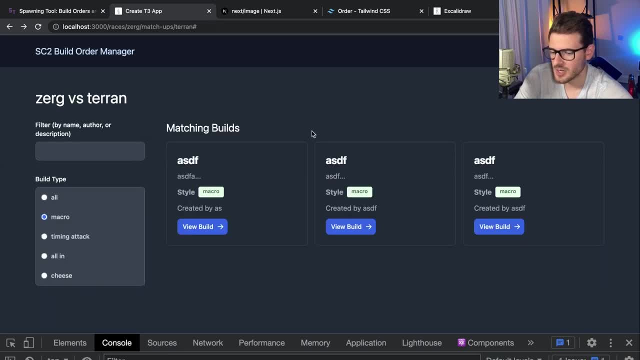 delete it from here because there's extra noise for the user. so that's how you kind of go about building complex software. it's all about, like understanding your user needs- what do they actually use, what do they not use? and you delete the stuff that's used by a very small 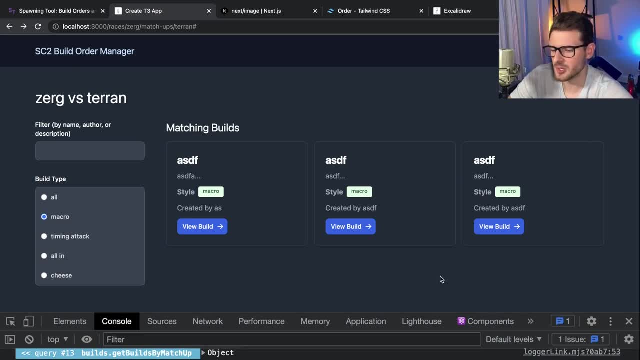 portion of users, and then also in terms of like the coding and the designing, can you design and code the the most minimal thing to get the feature working? and then you might say that, okay, you're going to code yourself into a corner because you're just going to add code that's sloppy. 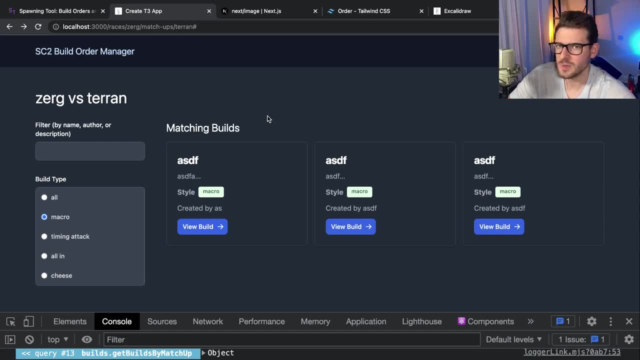 and it's not going to be extendable. but the point is is that when you get a feature down the road that requires you to change or modify or extend your current code, that's when you go back and you fact your code to make it that you know solid approach or to make it. 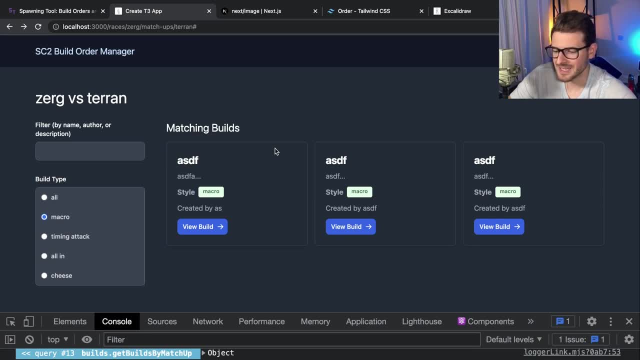 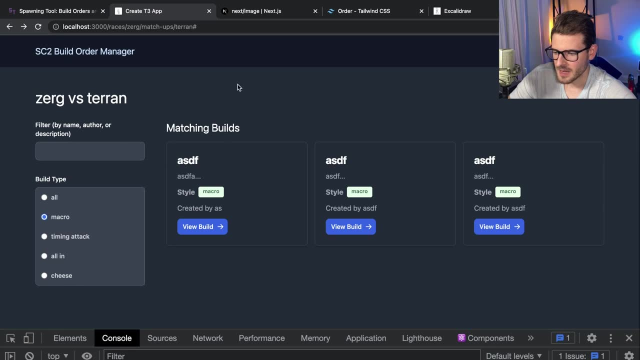 like design patterns approach to make it really extensible, make it really extendable and really modifiable and maintainable. But yeah, that's all I wanted to really rant about. I've met people who like to think about all the different edge cases when they're building code, And that's fine too. 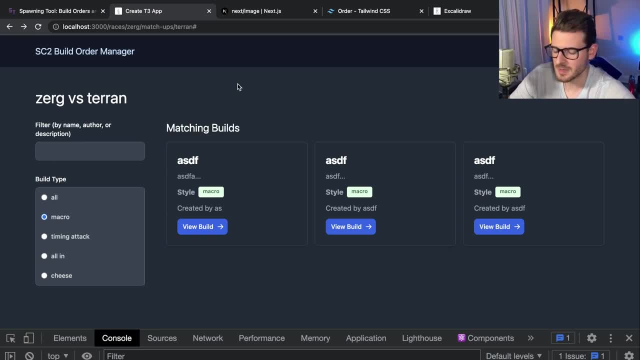 I think it's good to have. now. that's just my mindset. Again, there's different types of people. I have had people in my discord ask me like like a beginner in my discord whose professor is basically telling them to design this huge UML diagram or ER diagram of like 20 database entities. 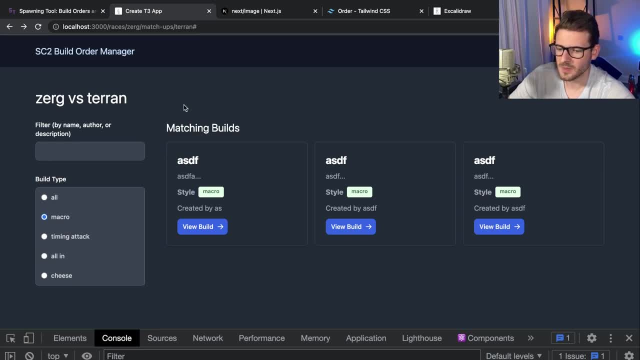 all from the get go And I was basically telling him there's really no point to sitting down and doing that Like. the real benefit comes from just slowly adding these features for your users and getting them to use it and slowly adding migrations and changing your database and 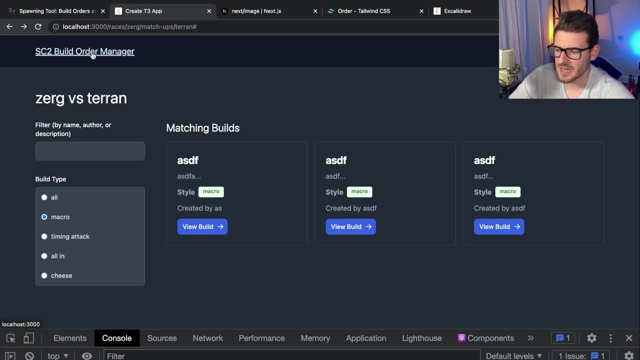 getting everything built out. There are teams who sit like would sit down and literally plan out every single page, like they'll plan out this page and they'll have like designs for this page and they'll have like designs for this page and they'll have.